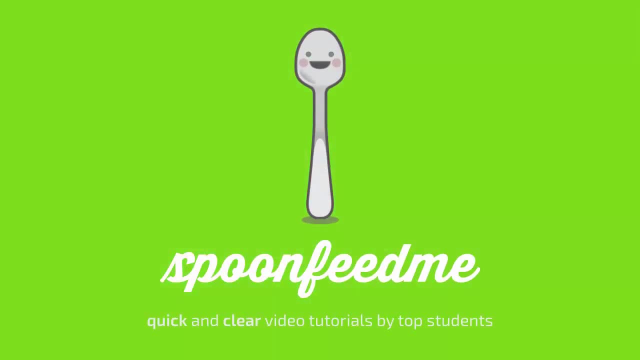 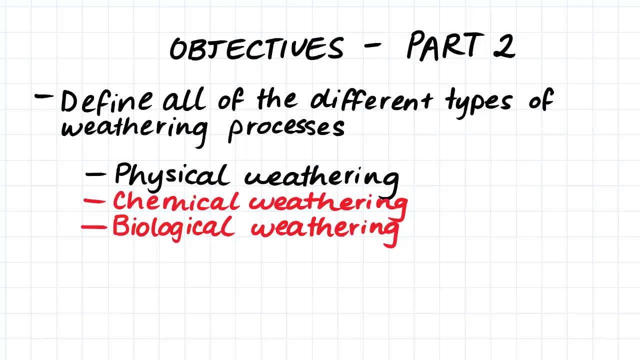 Hi guys, the objective of this video is to finish off defining all the different types of weathering processes. This is the second video of two videos in which we have been talking about weathering. The first video was all about physical weathering, but now we will be talking about chemical weathering and biological weathering. 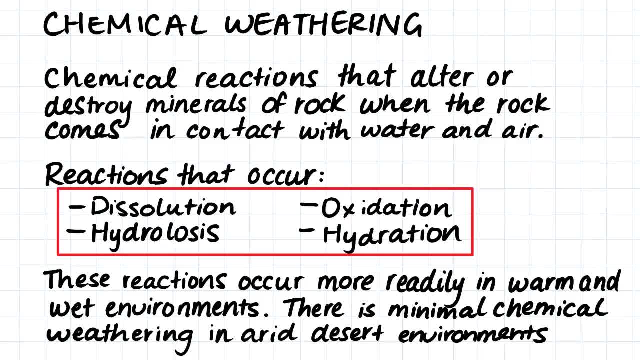 So firstly, just to define chemical weathering. Chemical weathering occurs when chemical reactions happen, and these chemical reactions alter or destroy the minerals of the rock. when the rock comes in contact with water or air, The reactions that occur include dissolution, hydrolysis, oxidisation and hydration. 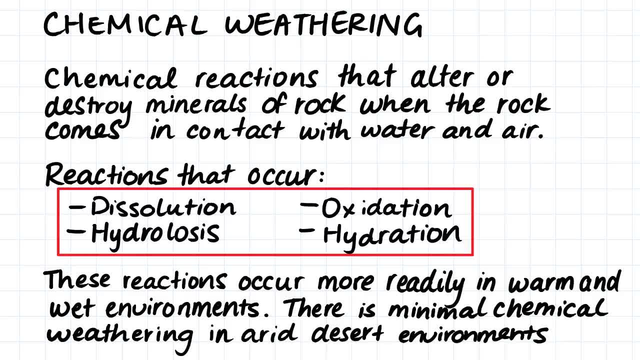 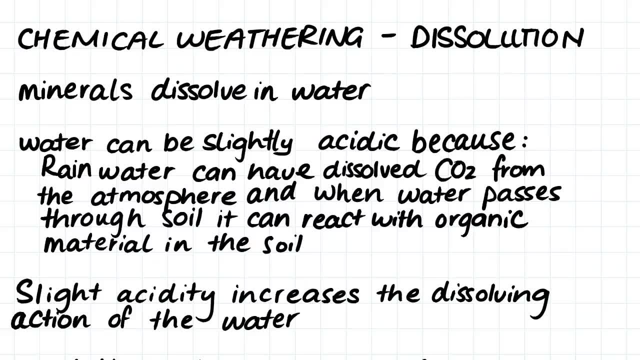 These reactions occur more readily in warm and wet environments, and therefore we can find minimal chemical weathering in arid desert environments. Firstly, we are going to talk about dissolution. Dissolution occurs when minerals dissolve in water. The water that comes in contact with rocks can actually be slightly acidic. 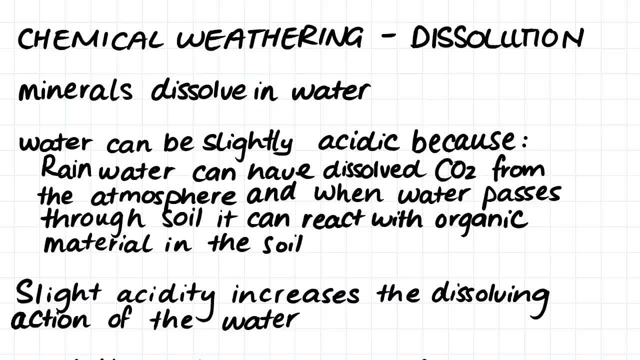 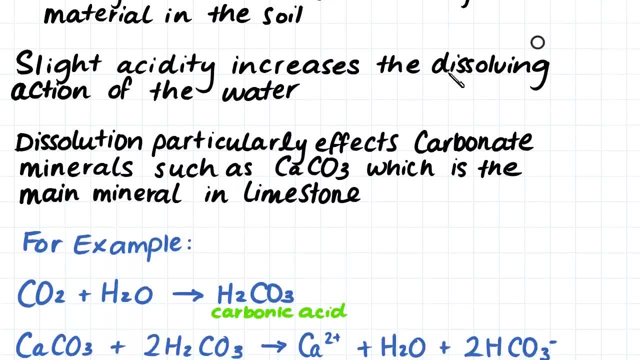 This happens because rainwater can have CO2 dissolved in it from the atmosphere, And when water passes through soil, it can actually react with the organic material in the soil and become slightly acidic. This slight acidity increases the dissolving action of the water. Dissolution particularly affects carbonate minerals such as calcium. 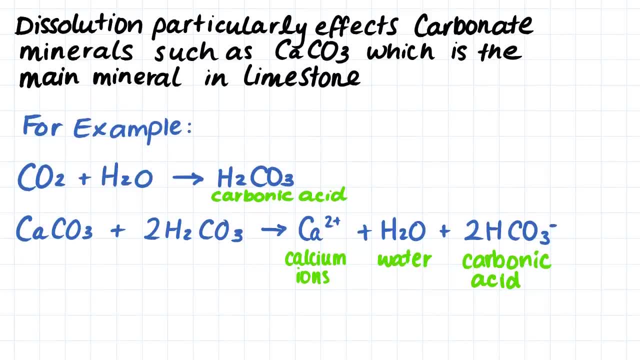 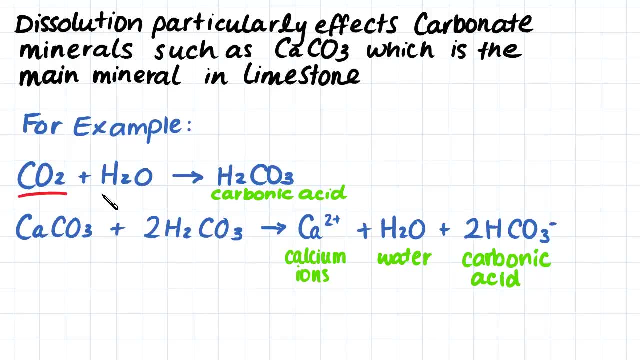 Calcium carbonate, which is the main mineral in limestone. One example of a dissolution reaction is this one here. Firstly, we have carbon dioxide dissolved in water. This produces carbonic acid. This carbonic acid then reacts with calcium carbonate and produces calcium ions dissolved in water. 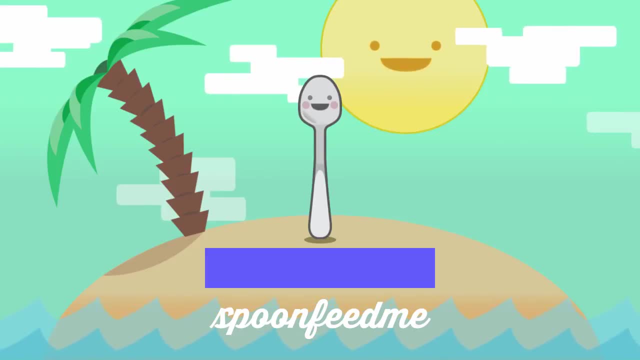 Calcium carbonate is the most abundant compound in the atmosphere and is the most expensive carbon dioxide of all, And it is the most rare carbon dioxide in the atmosphere. Calcium carbonate is very high in carbon dioxide and is usually found in the atmosphere, So basically, carbon dioxide can also be found in most places. Calcium carbonate contains carbonic acid and is a very well known product. There is also carbon dioxide in the atmosphere.